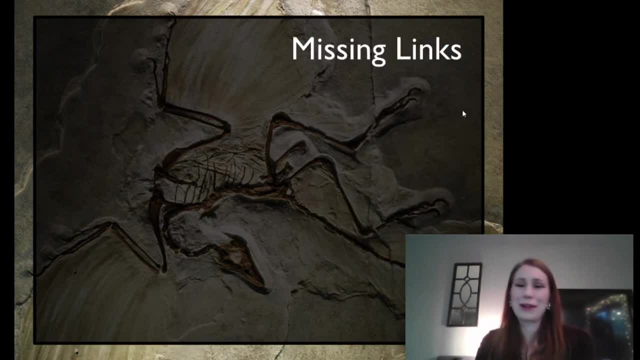 have looked like. Now there are missing links. The fossil record is by no means perfect, because the actual creation of a fossil is kind of difficult. It takes a lot of very specific conditions for those bones to calcify and turn into rock basically. So it takes a lot of specific. 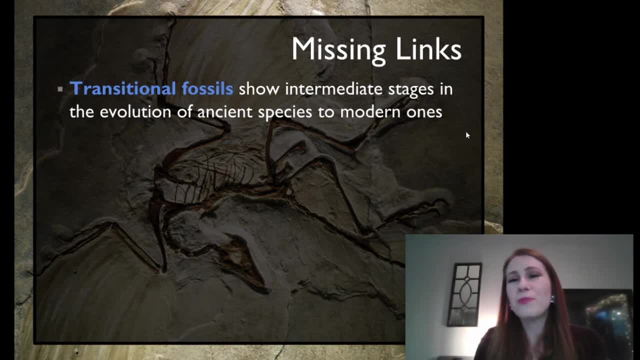 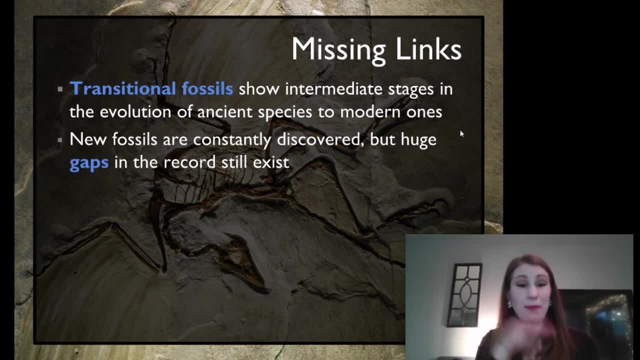 And I'll give you a couple of examples, But we're basically looking at those stepping stones in between an old species that probably doesn't exist anymore and a species that exists today. Because that's what we really want to see is: where did all these different species come from? 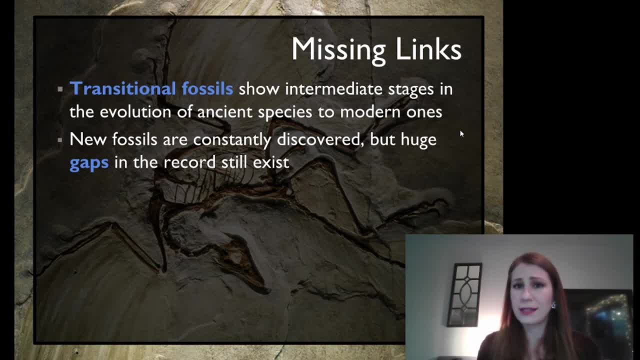 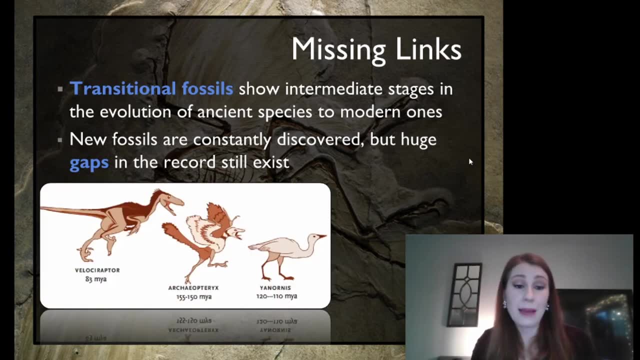 Who was their ancestor, And now new fossils are constantly being discovered. but we still have really big gaps in our fossil record. It's not perfect And that's just because we haven't had a lot of time yet. Now we do have some of these phases here between the Yenornis. I have no idea if I'm 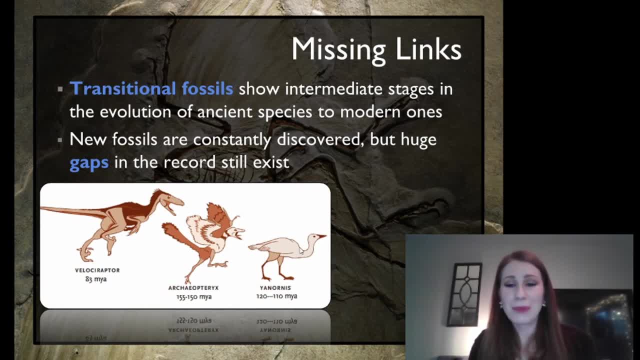 pronouncing that right, but I like saying Yenornis- It makes me happy- which looks basically like a really strange goose And this lived about 120 to 110 million years ago, So they found fossils for this species about that long ago. We also have a Velociraptor, which are of Jurassic Park fame. 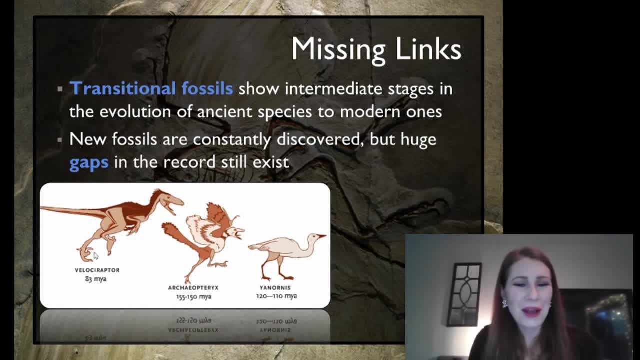 which was only about 83 million years ago, which might confuse you a little bit. I did not flip those around. The Velociraptor technically would be younger than the Yenornis, which is looking like a modern goose, So there's a little bit of confusion here. These do tend to have some. 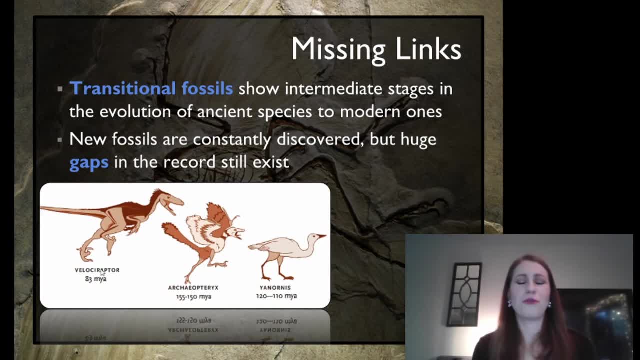 things in common, but we need to have more transitional fossils to really show us these kind of different phases, because these look like completely different organisms, even though they may share a lot of similar features. We also have the Archaeopterisks, like we see on the background. 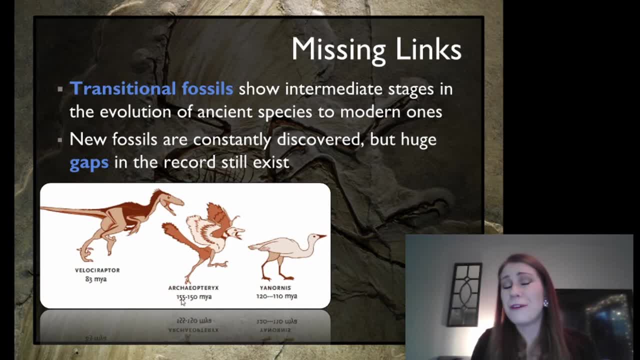 of our slides here, And that was about 150 years ago, So we have a lot of different things here. So what this may indicate to us- and again this is an indication- is that both the Yenornis, the kind of modern looking goose, and the Velociraptor may have been related to these. 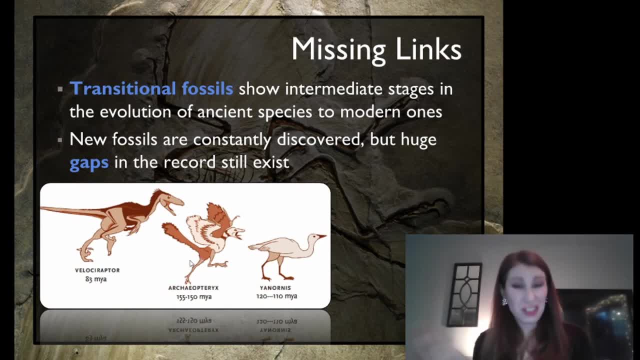 Archaeopterisks as its common ancestor, which is a little bit crazy, But that's why we need a lot of these transitional fossils to kind of visualize the changes that may have occurred to get from this kind of bird-like reptilian creature to the Velociraptor and this 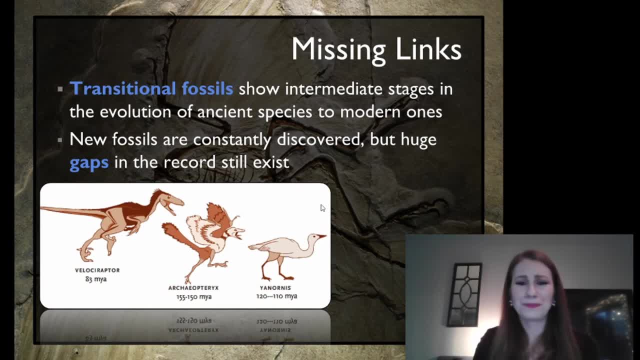 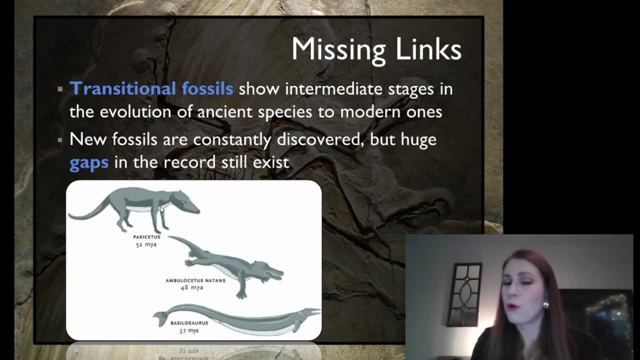 goose. basically, I'm going to call it a goose because it kind of looks like a goose. Now, sometimes it's a little more linear, We can see it a little bit better. We have the Pachycetus, which was a four-legged creature that kind of walked on land. 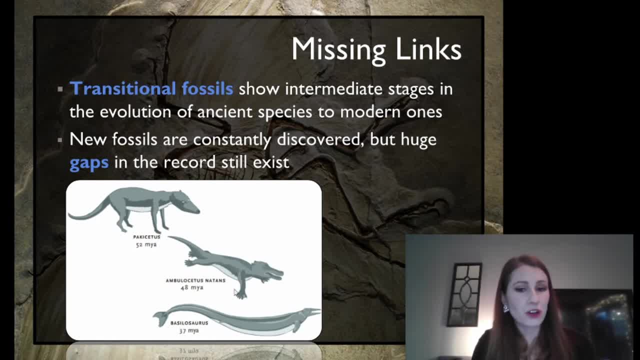 To the Ambulus Natans, which is going to have some webbed features but look very, very similar in the structure of the head shape, a lot of other bone features. And then to the Bacillusaurus, which looks kind of like a whale And you can see it's got tiny. 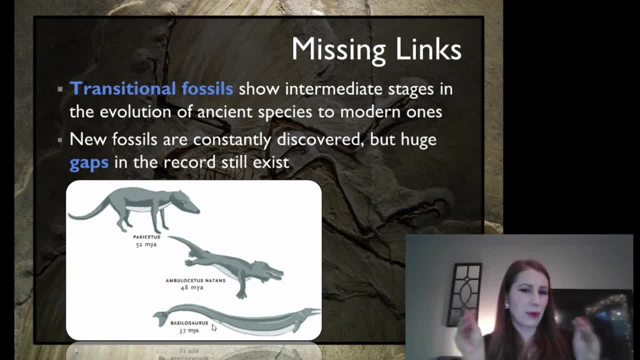 little. you probably can't see it, but there's tiny little backbones Slippers there that are pretty much useless at that point. So that's what we'll call a vestigial structure, And in modern whales you'll actually see the remnants of those bones. 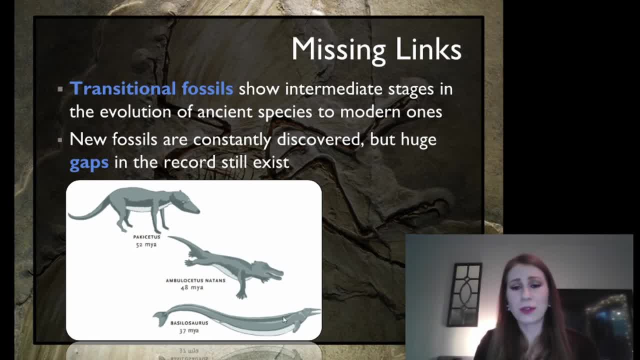 but there are no use for them. So it indicates that those are. what we have now are commonly known as whales, but they may have come from a land creature at some point. I mean, we're talking 52 million years, So it's kind of a long time for this change to happen. 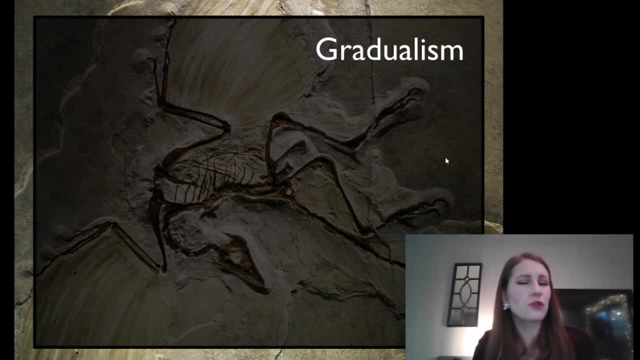 There are a couple of patterns by which the fossil record can be looked at. The first one we look at is called gradualism. This one is one that makes a lot of sense to me. It just kind of helps my brain. It makes my brain happy because it's showing us a slow, steady rate from something. 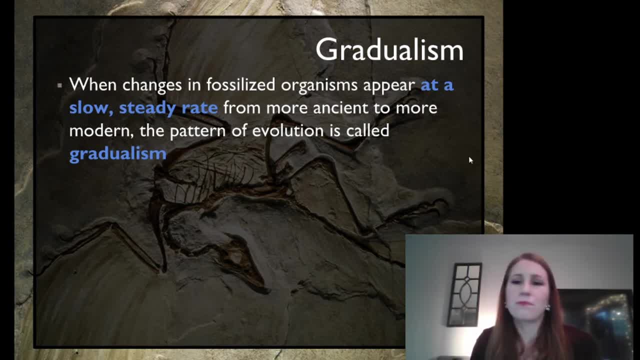 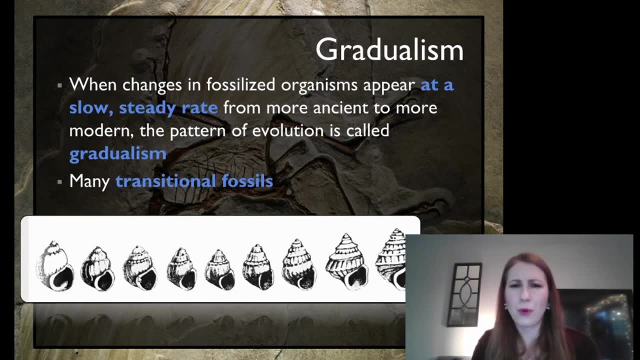 that's more ancient to something that's more modern. This pattern, gradualism, it makes sense. It's gradual the change. There are lots of transitional fossils. So here let's look at an example. We start with this older version, much smoother, of a shell and whatever creature would. 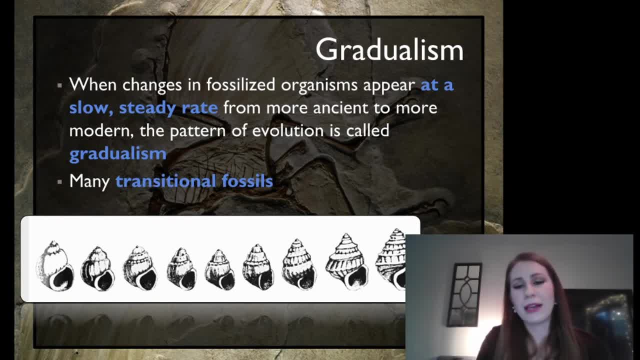 live inside of there. This is kind of an illustration, And over time it shifts to a different type of shell. So this would be an example of gradualism, something changing very slowly over time. We can tell how it got from one thing to another thing, because there's many of 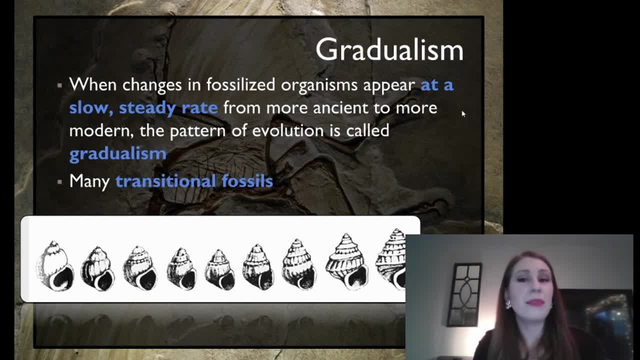 those in-between steps or transitional fossils found, And this does occur with some of the things that we see, but not everything. So that's why it can be tricky to always try to apply gradualism as a pattern. It doesn't always work. The second pattern is called punctuated equilibrium. 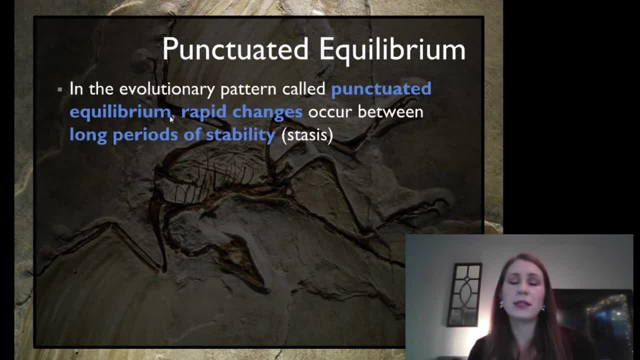 This we see quite a bit. It's basically a a pattern of rapid change, so quick change followed by a period of no change, stasis. So it could be due to a catastrophic event: Something causes a specific type of organism to survive better And then it stays that way for a long time. Or it could just be that we don't. 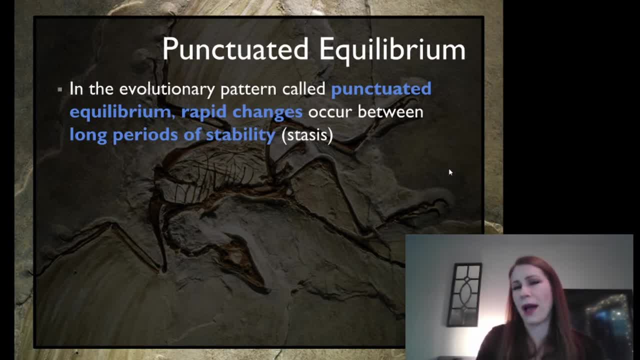 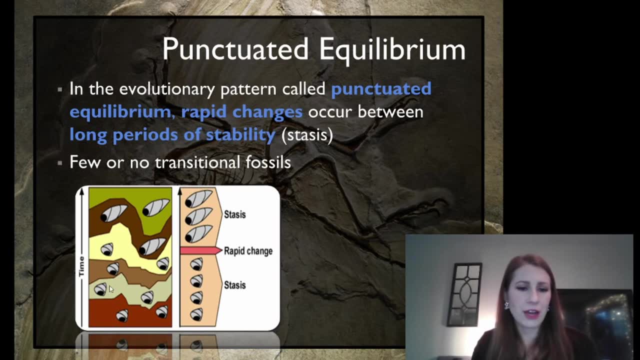 have the in-between fossils and we can't call it gradualism because we don't have transitional fossils. So here is the example picture for this one. So we have what we see over here found in the small입 layer. It's relatively small. This one's a small from the early 20th century. 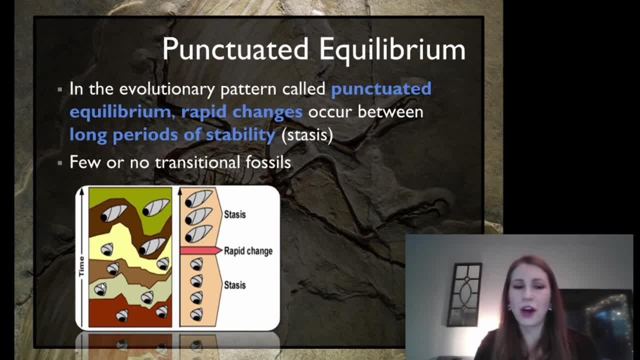 So this would be older, This would be younger rock layers at the top. We see these, the small shells. for some reason they were good to go for a long period of time. There weren't that many. You can see right here stasis, So it was all small shells. Then, right around this time, we see that there may. 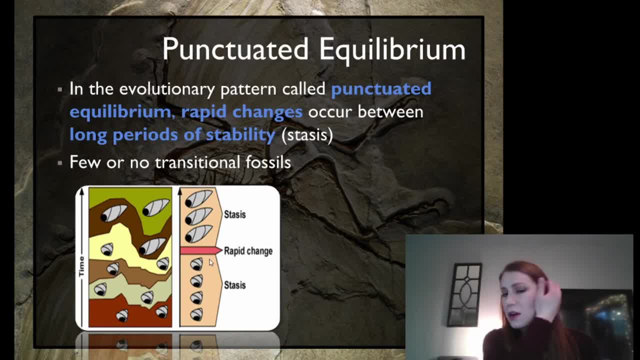 have been a mutation and these longer shells started to appear as well. Then something happened- Probably larger shells. This is punctuated equilibrium because it's stasis followed by a rapid change, followed by more stasis. So punctuated means like something that's been popped in the middle and 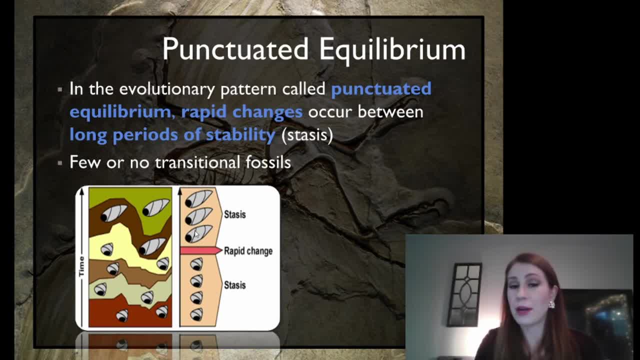 that's our rapid change. that's been popped in the middle, And then equilibrium means it stays the same, So that's why we have stasis as well. Now, in all actuality, our fossil record is probably a combination of the two things. It's really hard to just fit it into one pattern So punctuated. 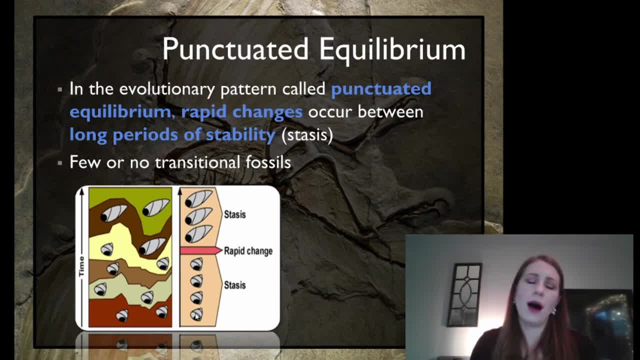 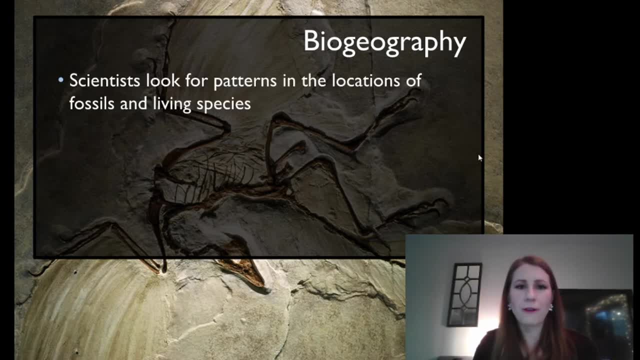 equilibrium and gradualism are probably all part of our fossil record and how evolution has occurred as a pattern. Biogeography is something that we can use to help us look for patterns in the locations of fossils and living species as well, But we're looking at where these fossils 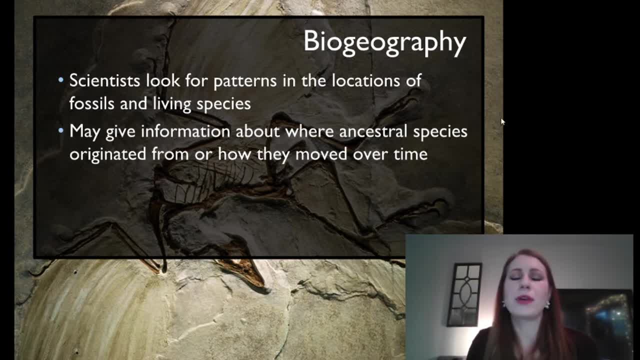 occur location-wise on the globe, So they can give us information about where ancestral species- so ancient species- may have come from or how they may have traveled over time. So species don't just stay in one place. Lots of animals tend to migrate, whether they need new food sources or they have to travel because there are natural. 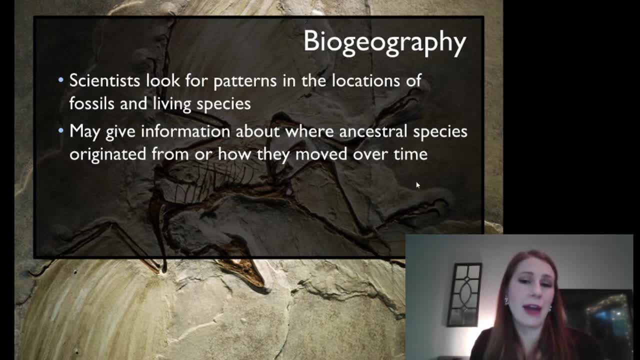 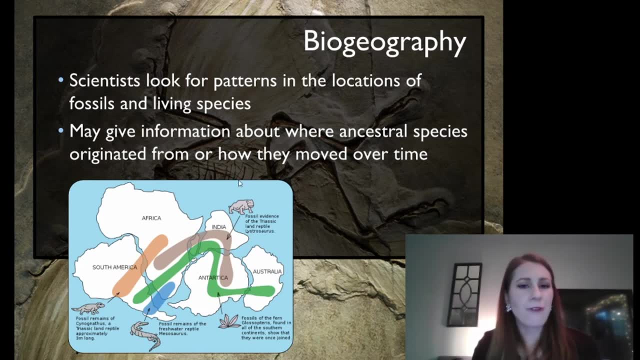 disasters, making them move For whatever reason they may have moved over time. And we can see in pictures like this- and I'll make it much larger in a moment- that we have fossil evidence of specific creatures on different continents in our globe. 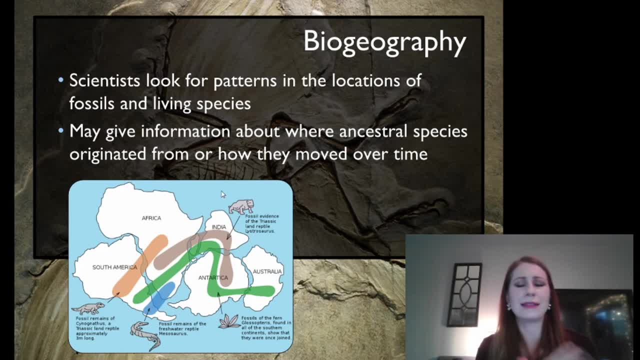 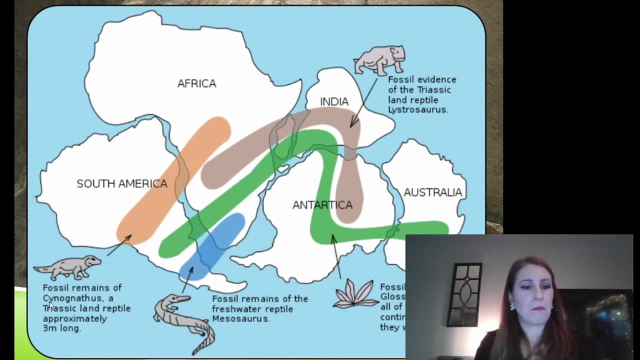 Which is kind of crazy, because they're separated by oceans and some of them are not water-dwelling species. So land animals somehow crossed between these continents millions and millions of years ago. So let's take a closer look. Let's have an example here of the Cynognathus- Again, not a. 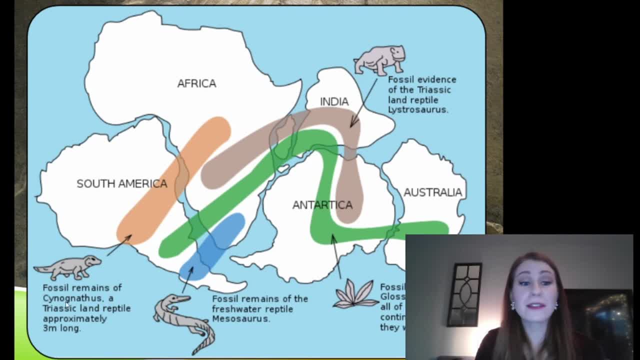 pronunciation that I'm super used to, but I'm going to go with Cynognathus, And that is a Triassic land reptile. So it's a small-ish land reptile. Three meters long is about nine feet, So I'm thinking something similar to a. 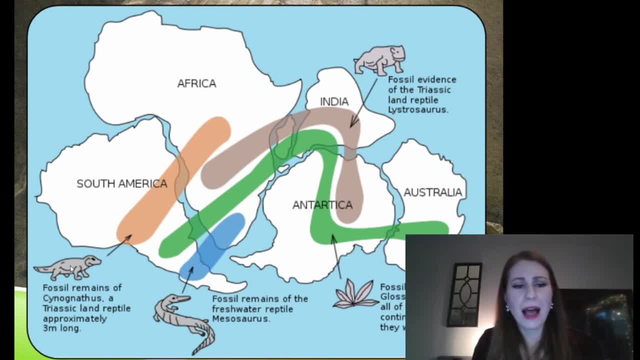 alligator size. So we have that here. However, it's a land reptile, So it did not live in the water, And remains of it are found in South America and Africa. This was before we had boat travel, before we had plane travel, So that animal did not get on a plane and fly to Africa. 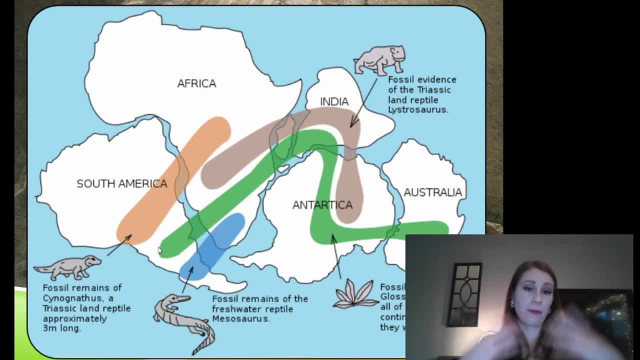 It indicates to us that our Earth at one point had a much, much closer structure with our continents. We call that Pangea. It would be much easier for this land reptile to have crossed on a land bridge between South America, what is now South America. 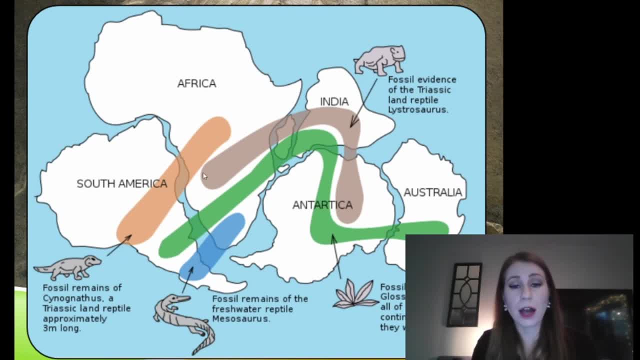 and Africa at some point. So we use a lot of these different kind of markers to show how the structure of the Earth may have been millions of years ago. It also helps us to see that these animals were capable of moving long distances, Especially if their ancestors are found in different continents today, Because you may have 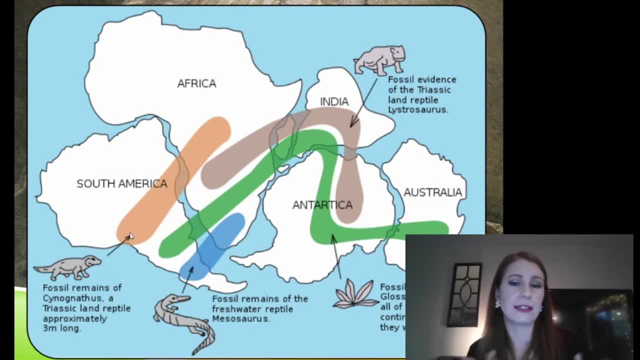 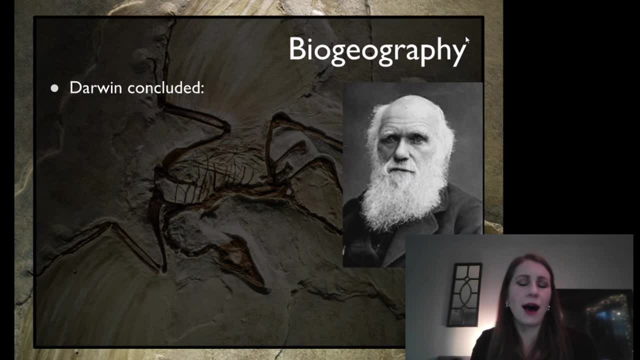 some very closely related species found on completely different sides of the globe due to this Pangea-like Earth structure. Now, biogeography was something that Darwin studied a lot. Charles Darwin, He was known as the father of evolution, natural selection in some ways, And essentially, 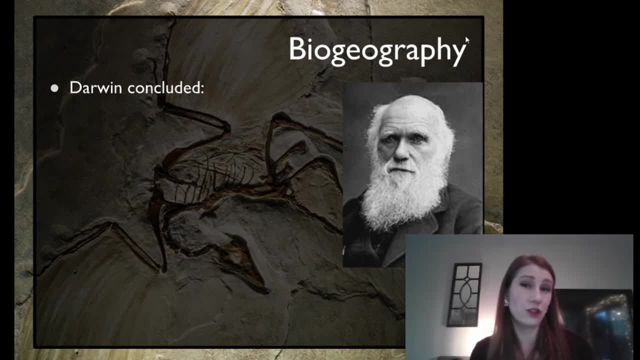 he was an explorer who traveled and made a lot of observations Back in the 1800s, I believe. Don't quote me on that again. History not my subject, But you can look up Charles Darwin if you want to, And some of his conclusions about biogeography were pretty. 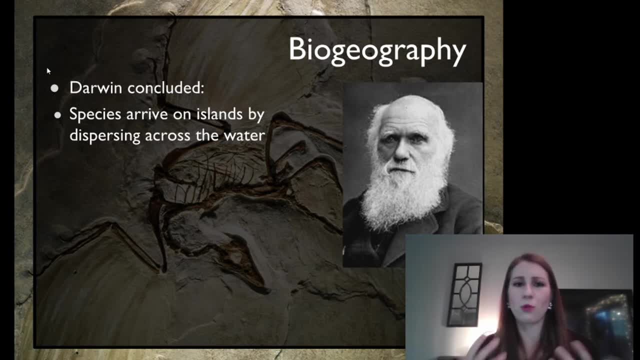 simple, At least they seem that way to us. now. Species arrive on islands by moving across the water. That makes sense. If you don't move across water, you can't get to an island. So that one I was like. oh gotcha, Darwin Makes sense. Dispersal from nearby areas is more likely than 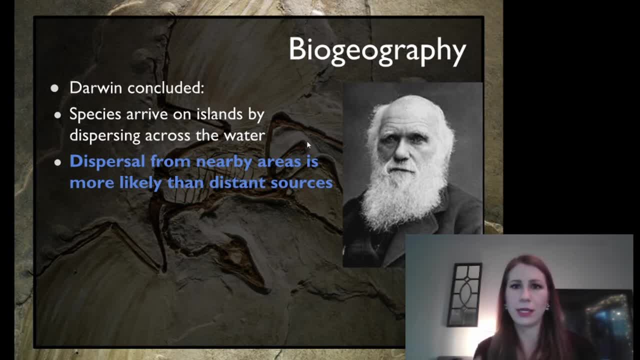 distant sources. This also should make sense. Let me kind of deconstruct that. It means that, for example, if we are on the continent of North America and there's an island about five miles off the coast, it makes sense that a creature or an organism could come from. 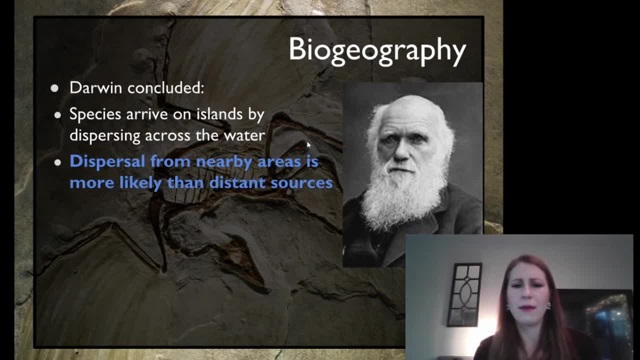 North America to that island because it's five miles away. It's much more likely that happened than it coming from Australia, way further away. You think that animals are going to travel a much shorter distance than a longer distance if given the chance. So we're looking at them arriving from. 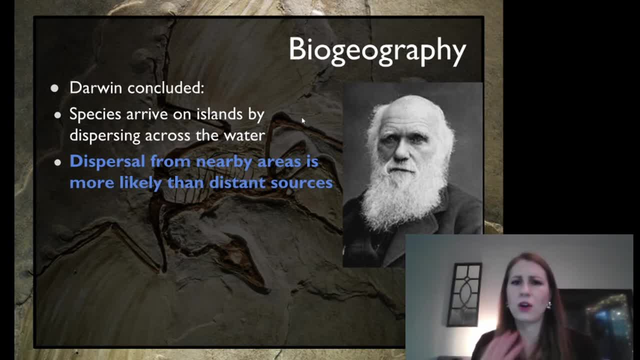 closer Areas. So again, this should make sense And I'll go over that again. That's kind of a tricky one. Species that can fly, float or swim can inhabit islands. So this again: if you can fly, of course you can get to an island. If you can swim, 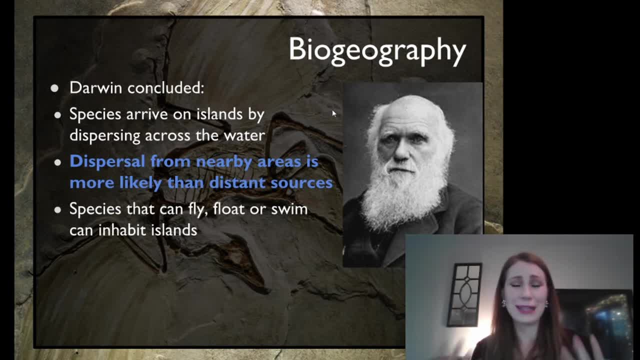 you can get to an island. If you can float, a lizard could theoretically get on a log and float over to an island. It's not ideal, but it can happen. It's not something that would be happening all the time, but this is definitely something that could occur, And a lot of times those 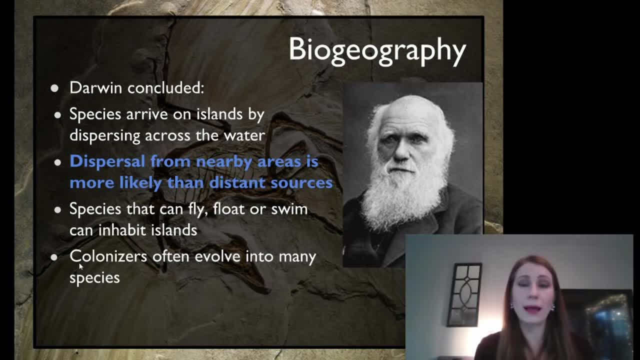 colonizers, or those first organisms that come onto a new island or a new land area. they can evolve into many different species, So you can have one common ancestor that is highly related to many, many, many new species that you see millions of years later. 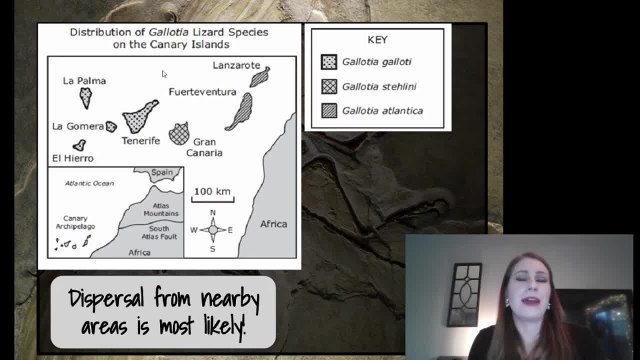 Let me kind of highlight this for us. So if we look at this picture, we see that we've got in this small one here. we've got these islands, the Canary Islands, We have Africa here, And then over here we see the tip of Spain, which would be 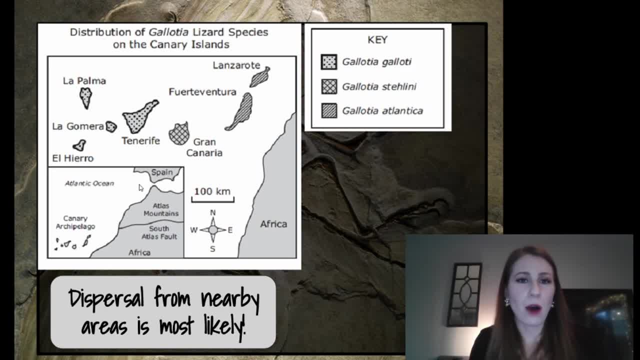 Europe. So if we're thinking about where these lizard species most likely came from, because lizards don't just appear on islands out of nowhere. islands are volcanic, so they can't just appear in a volcano, They have to come from somewhere already. 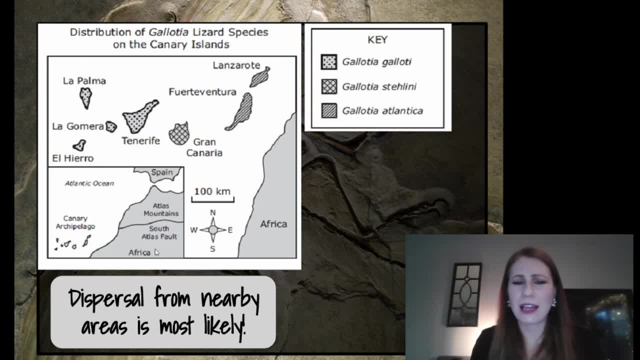 established. So are we going to think that it's coming from Africa or Spain? What would be more likely? If we look at this here, Africa is fairly close to these islands- I mean, 100 kilometers is fairly close, I guess- whereas Spain would be thousand or so kilometers away. 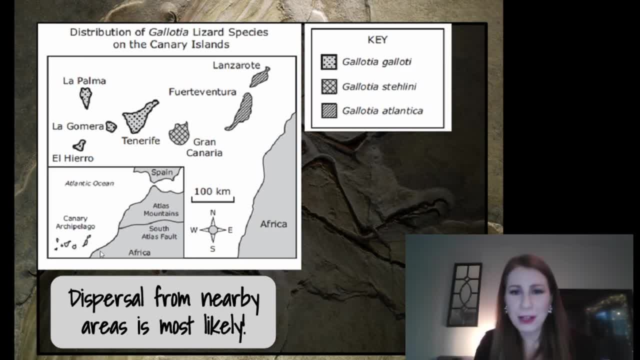 probably several thousand kilometers away. It's much more likely that these lizards originally came over from Africa than it is that they came over from Spain, because lizards don't swim very well, So those lizards would have a much harder time traveling to the islands from Spain than 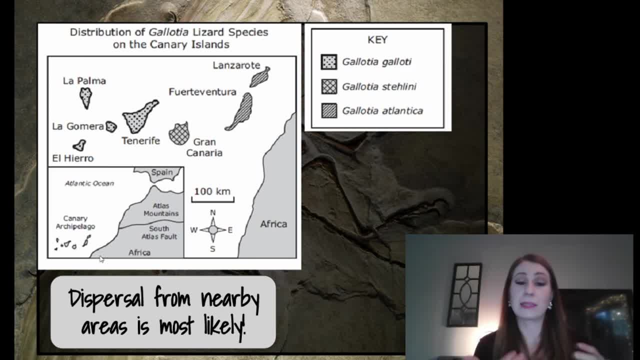 they would from Africa. So that's what we mean by dispersal from nearby areas- is most likely. It's much less likely if they were to come to the islands that are over the coast of Spain. So if we look, less likely that they traveled from Spain all the way to those islands. 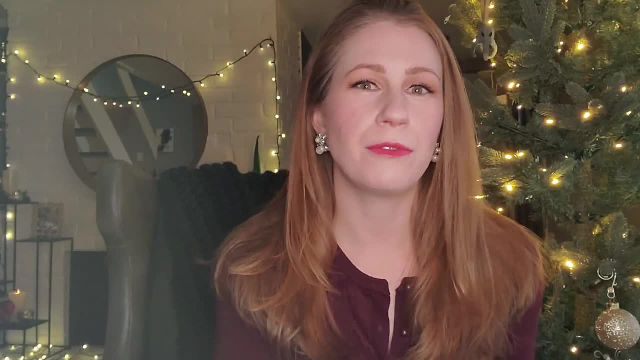 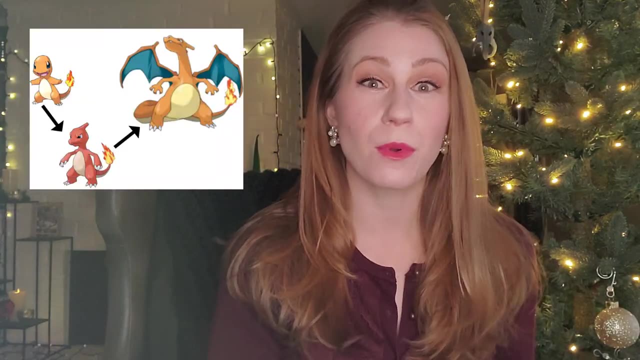 Just doesn't make a lot of sense. Let's review what we've learned so far about the fossil record and biogeography. First off, when we talk about evolution as a concept, it's important to remember that we're talking about change over time. 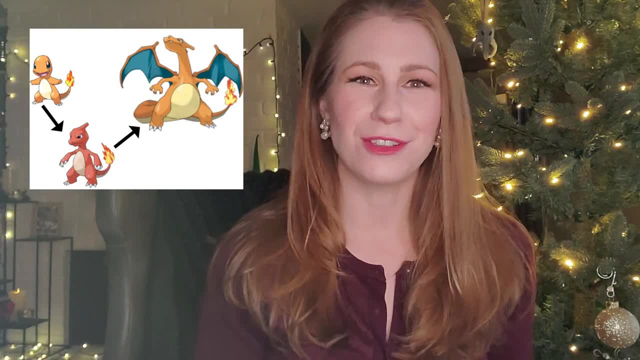 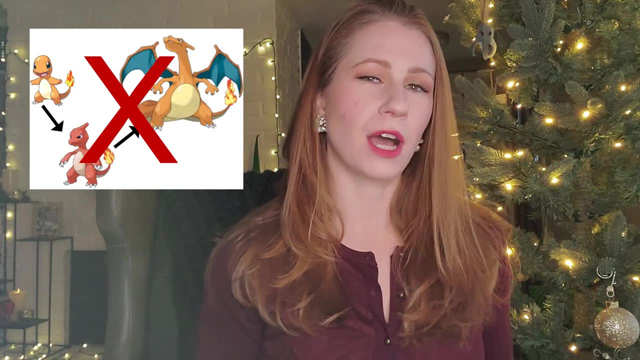 Now time being millions and millions of years and change, being in a population of organisms, not a particular individual. As much as I might like to, I do not evolve over time like a Pokemon. it would be really cool, but I just don't. 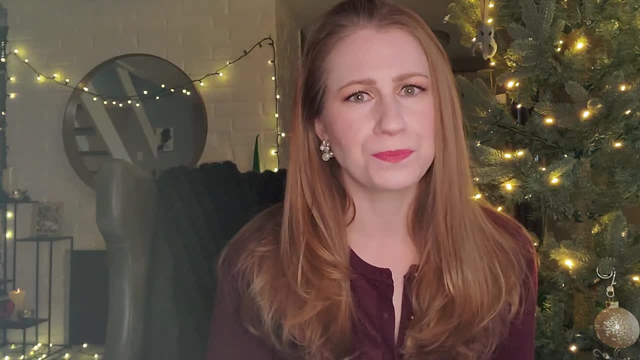 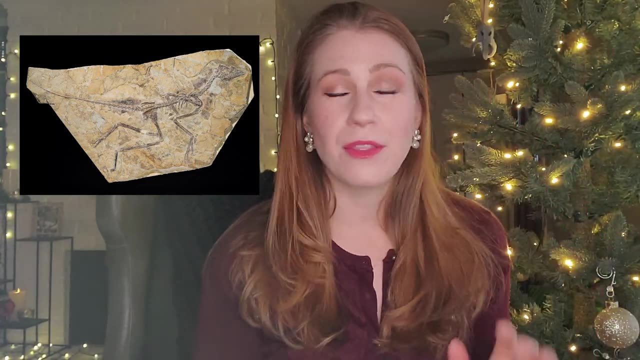 I develop and grow, but it's different from evolution as a whole. Now, fossils give evidence of change over time, but it's not a perfect picture. We can have gaps and there are a couple of patterns that fossils typically fall into. 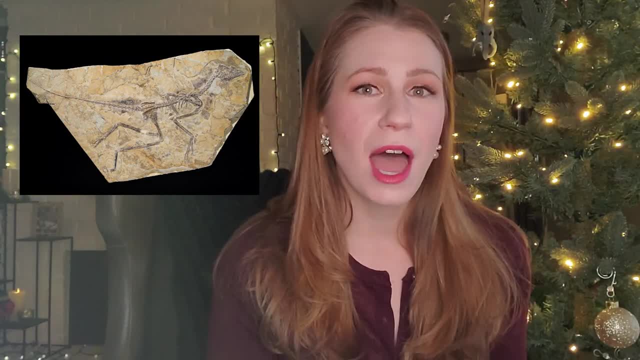 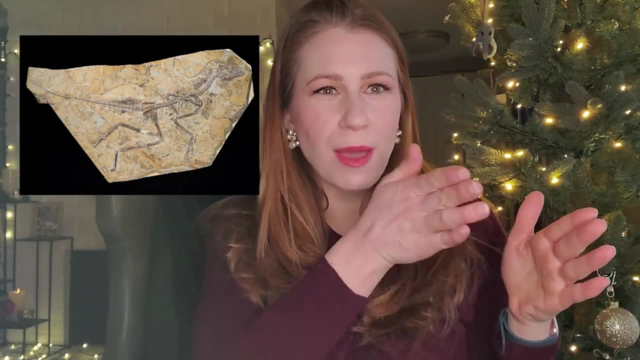 The first pattern fossils can fall into is gradualism, and this occurs when you have many transitional fossils and you start from one clear picture of one organism and you have many fossils in between, leading to a clear picture of a second organism, respectively. 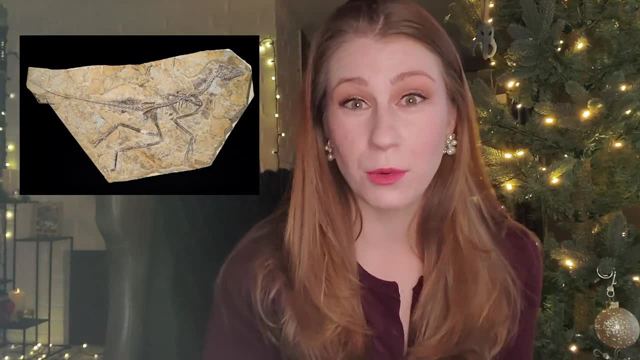 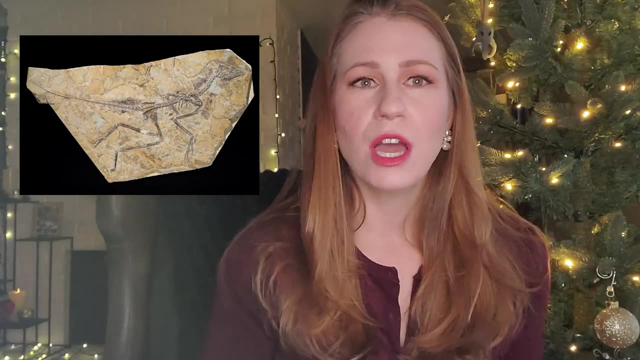 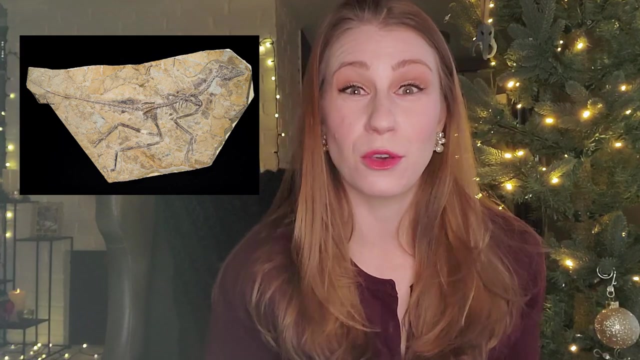 This is a pattern of long periods of stasis or no change, followed by periods of very rapid change. So you'll have nothing for a while and then something will happen and change, and then nothing will happen for a while. So you may not see those transitional fossils that you see in gradualism.